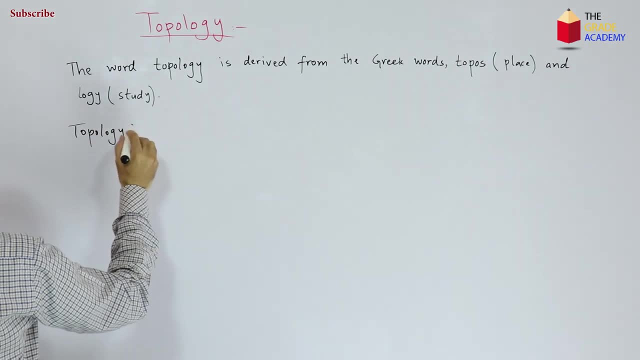 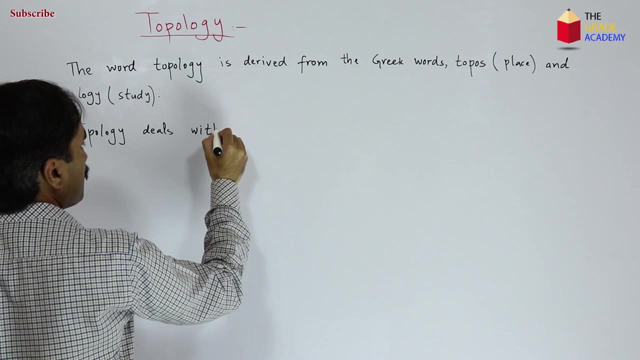 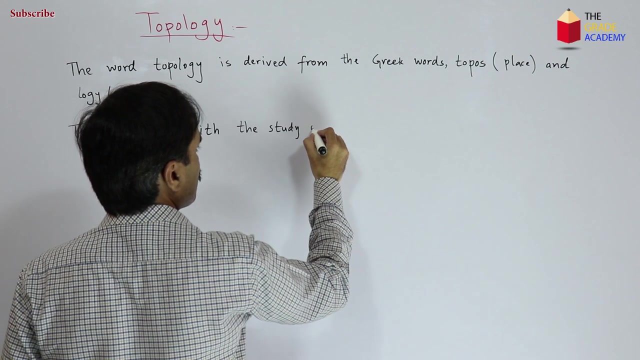 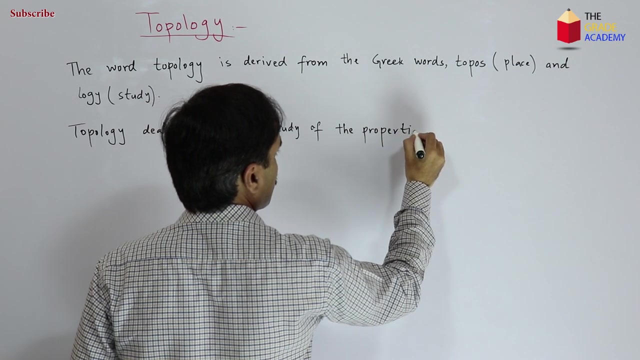 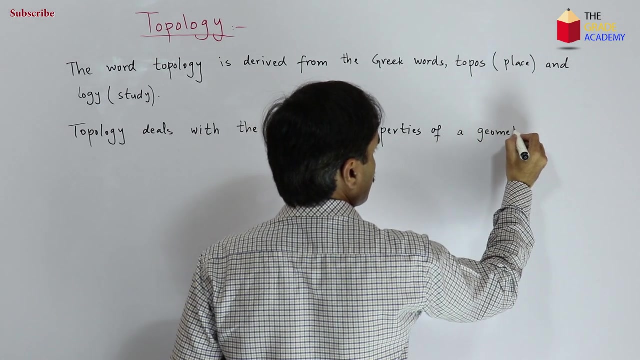 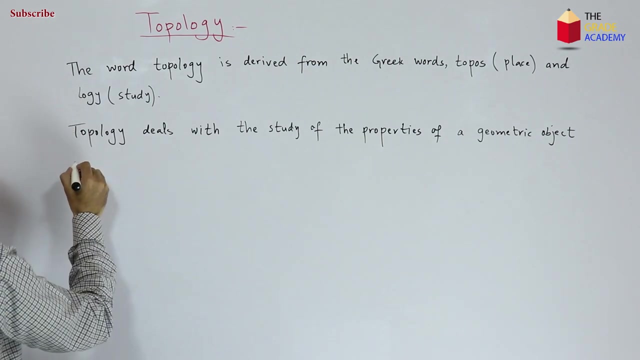 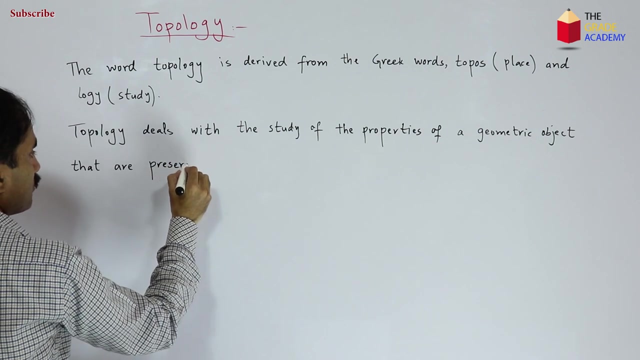 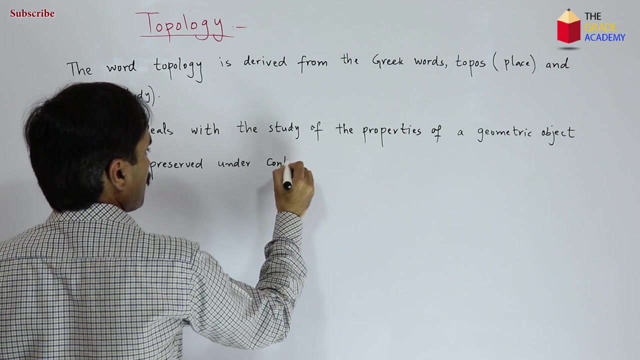 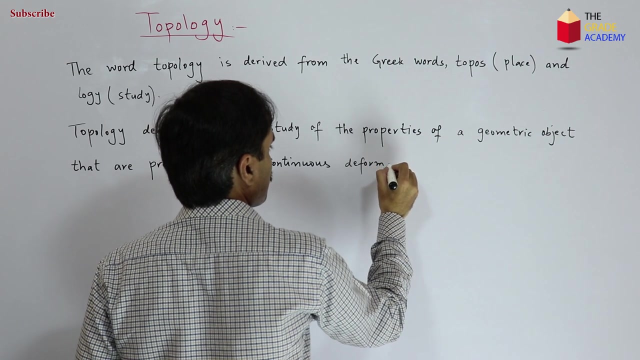 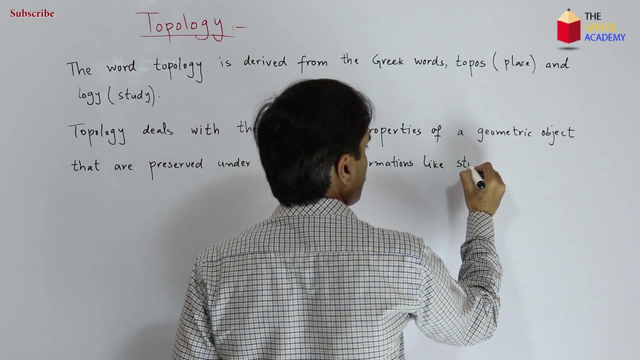 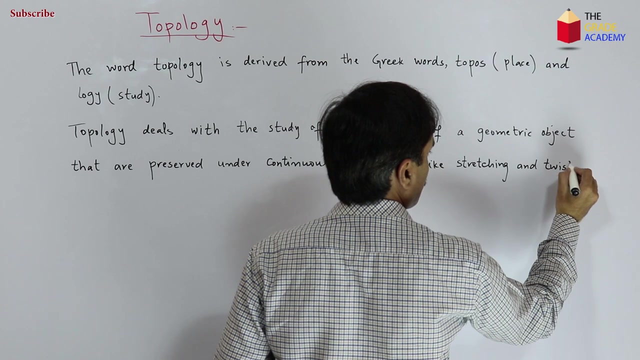 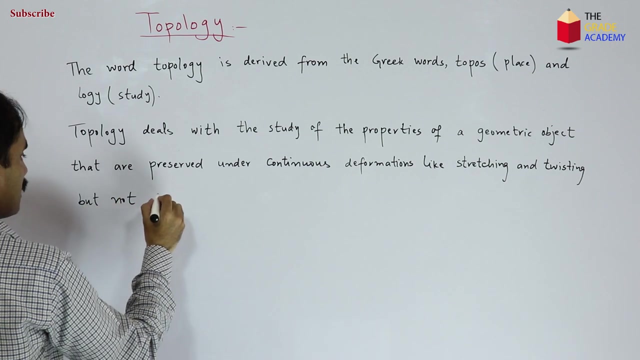 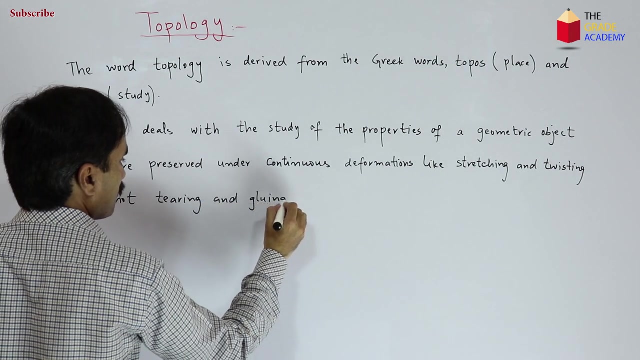 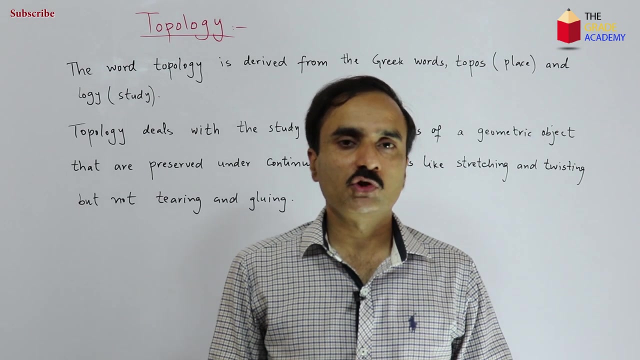 So topology deals with the study of the properties of a geometric object that are preserved under continuous deformations, like a stretching and twisting, but not tearing and ballooning. so topology is about all those properties of a geometric object which are constant or preserved under continuous deformations. 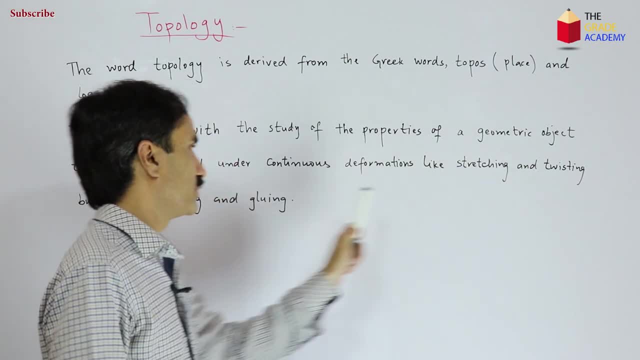 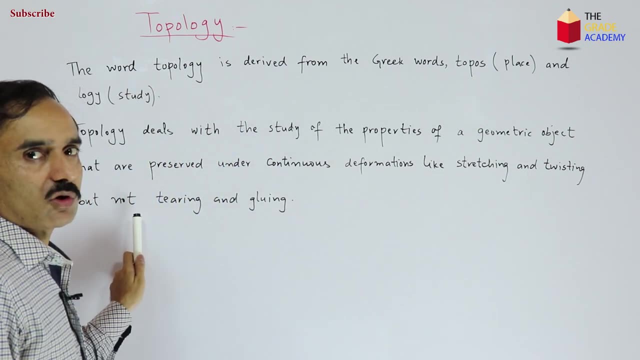 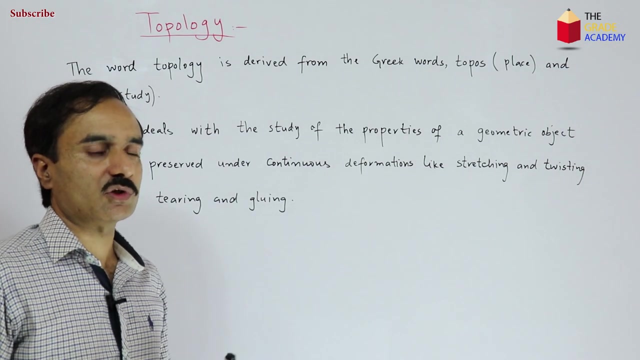 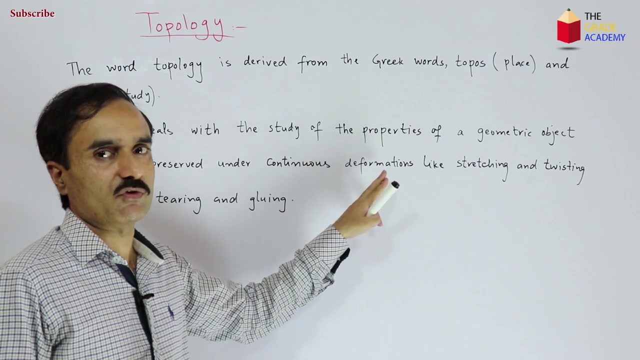 so topology deals with the study of properties of a geometric object that are preserved under continuous deformations, like stretching and twisting, but not tearing and gluing. so topology is about the deformations of shapes or objects, but that deformations have to be continuous deformations. so here the deformations have to be continuous deformations. 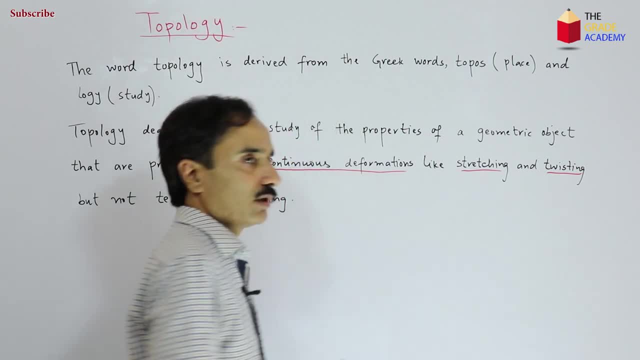 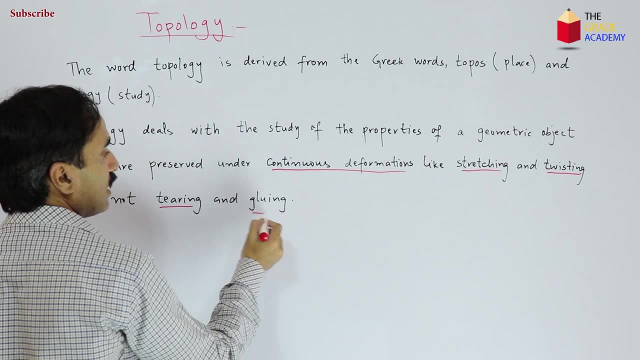 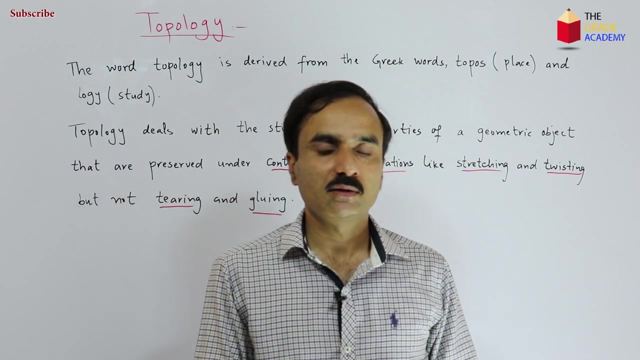 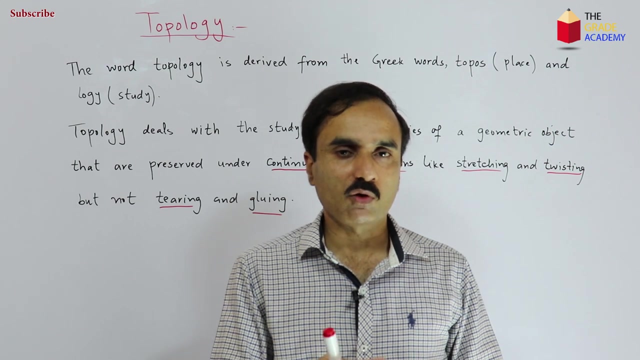 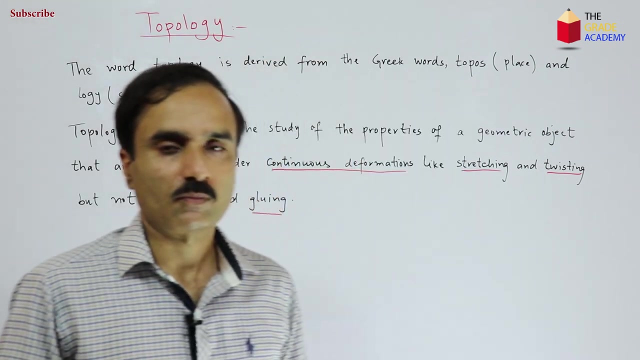 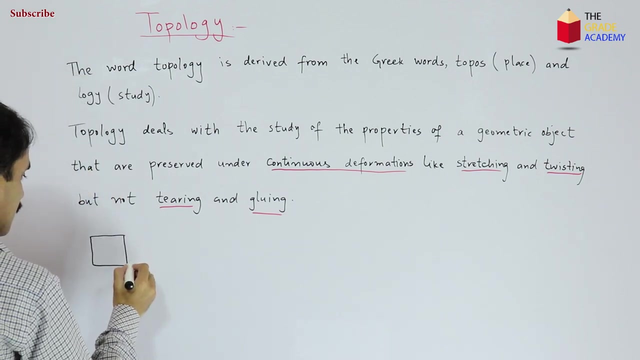 like stretching and twisting, so the transformations cannot be discontinuous, like tearing and gluing. so when? so? topology discusses how an object can be deformed into various shapes by the use of continuous deformations. so this is the main goal of topology. for example, a square can be deformed into a circle. 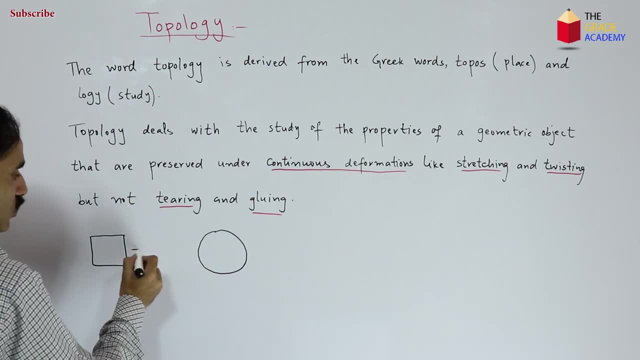 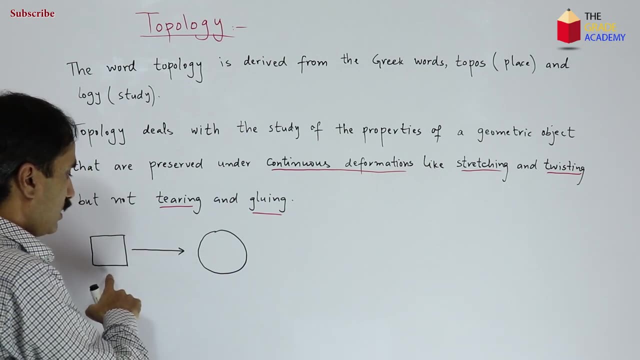 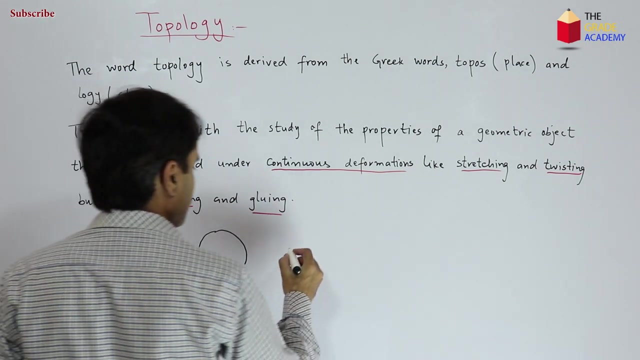 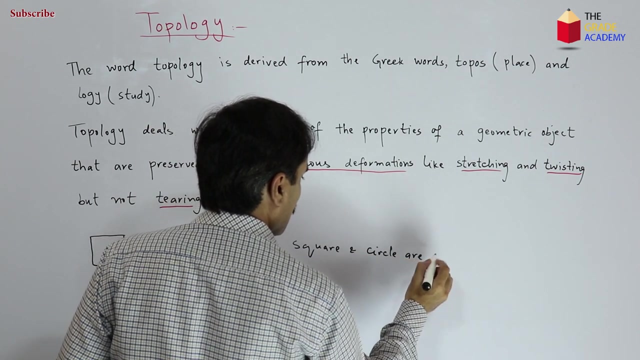 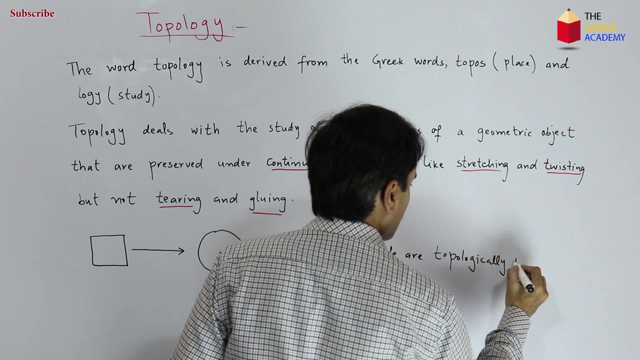 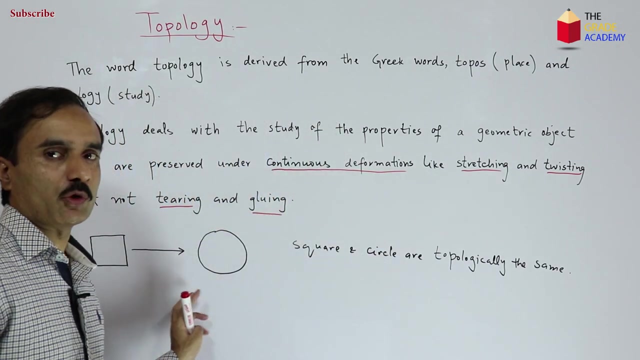 without breaking. so a square can be deformed into a circle without breaking. so this is a continuous deformation of a square into a circle. and we say that square and circle are topologically the same. so hence square and circle are topologically the same thing, or they are said to be topologically equivalent. 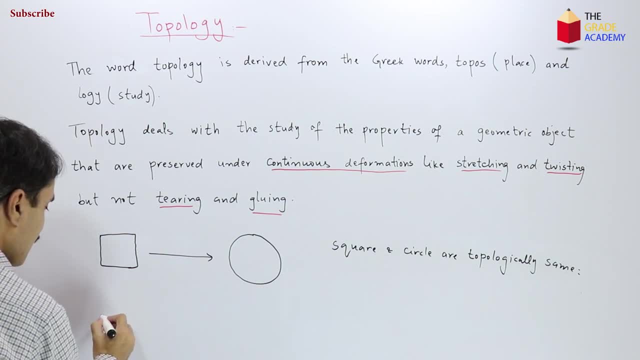 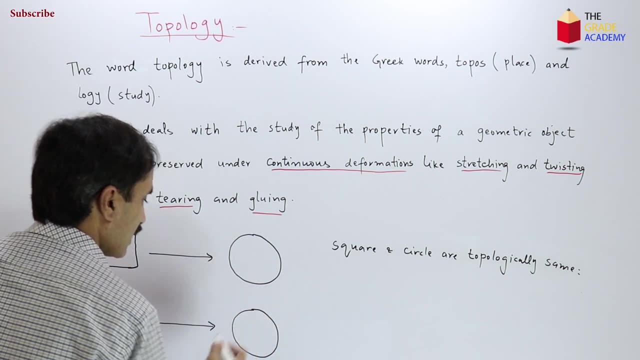 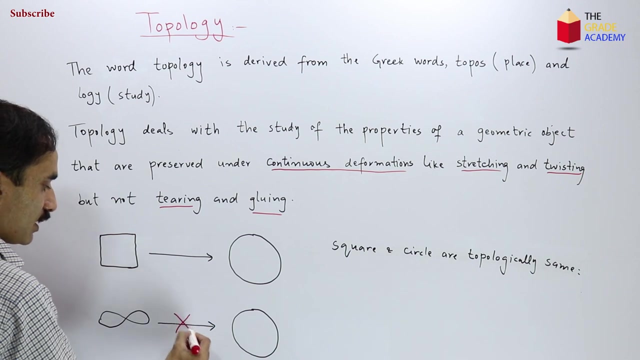 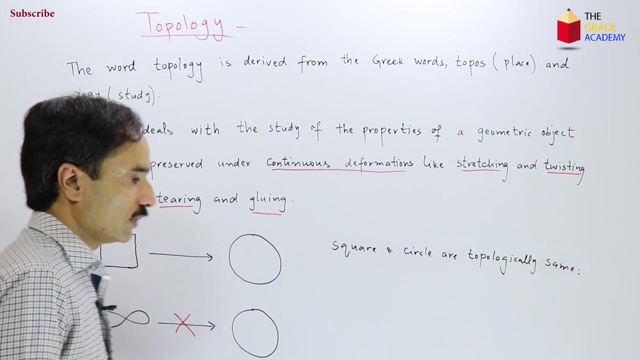 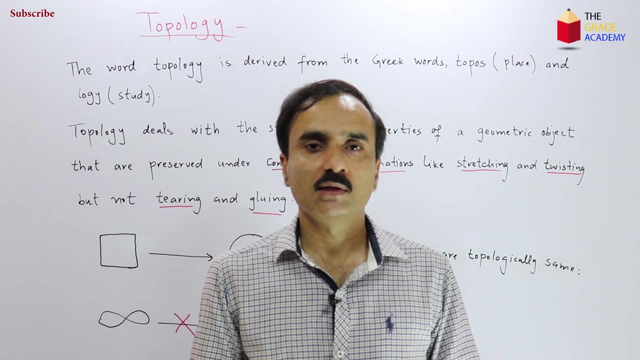 but here, if we consider this shape, the figure eight, and how about its deformation into a circle? so now we will see that this figure cannot be deformed into a circle without breaking. so two objects in topology are said to be the same if one can be deformed into another. 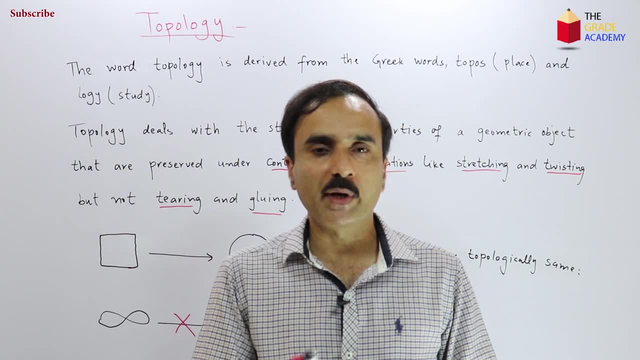 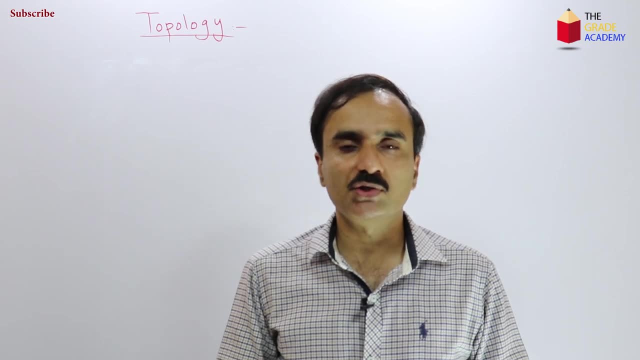 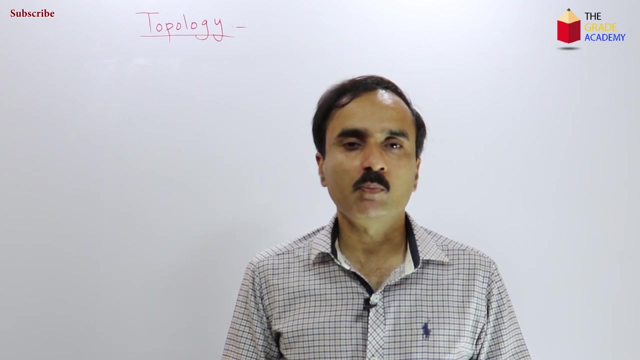 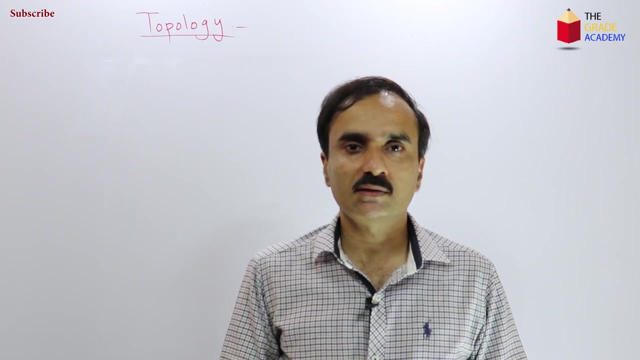 by a continuous deformation or without breaking or gluing or tearing. topology is sometimes called rubber-sheet geometry, because objects can be stretched and contracted like rubber but cannot be broken, is not the study of ordinary geometry. It doesn't care about length, volume and angles. 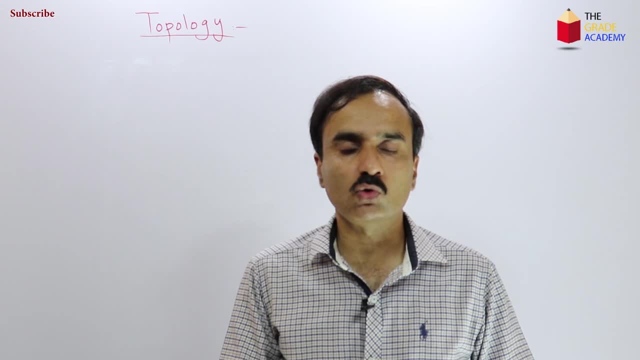 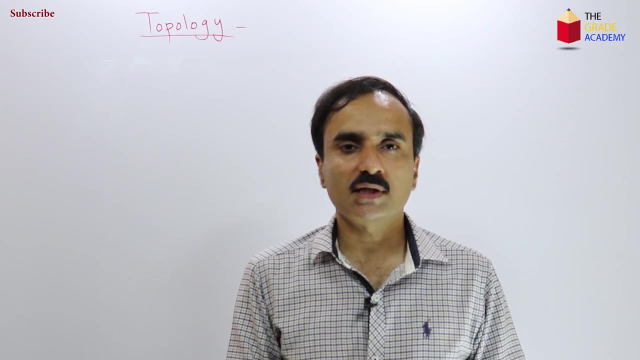 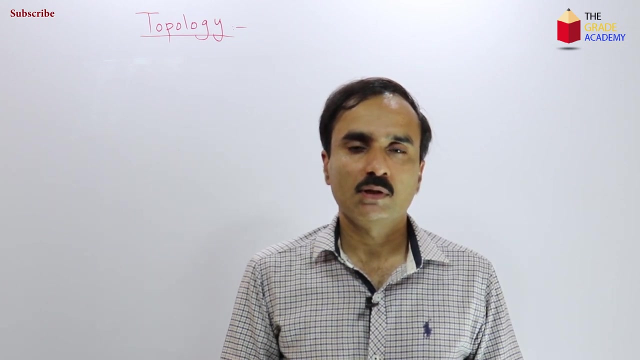 So its studies about shapes is sets or groups, So every shape is a kind of a set or a group, So it is a collection of properties. So as long as these properties are the same, the object is the same, no matter how it looks And the continuous deformations that we consider. 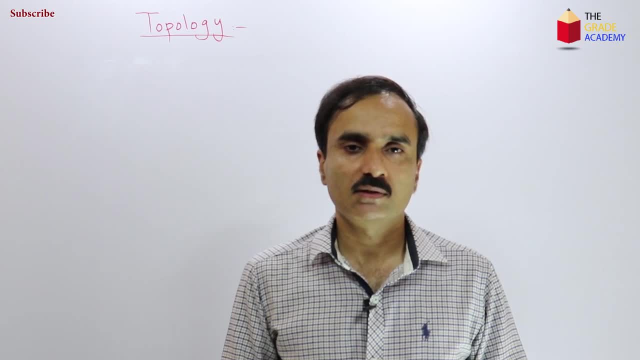 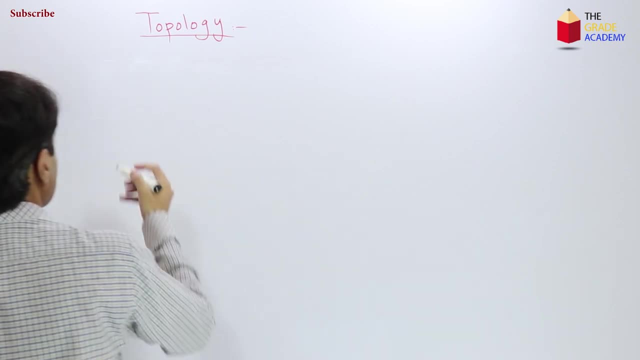 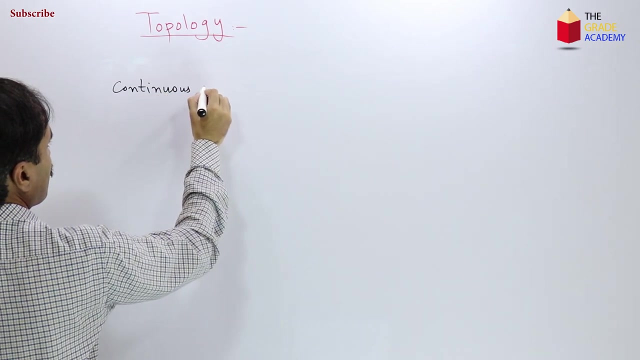 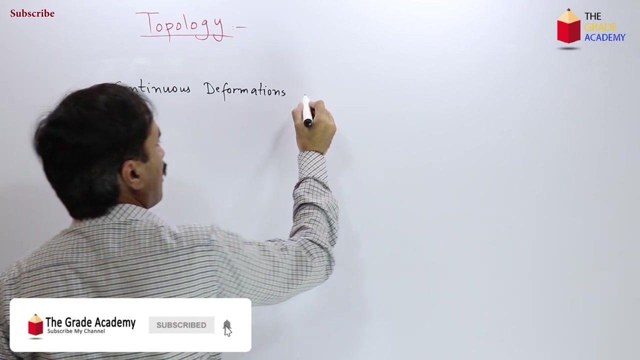 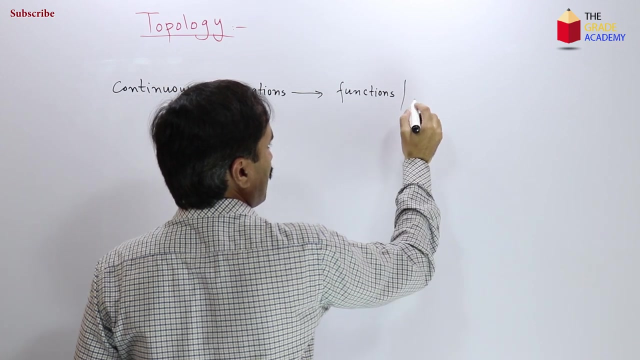 in topology, they are basically functions. They are continuous functions and they are called homeomorphisms. So the deformations are continuous deformations, So the continuous deformations are basically functions, what we could call homeomorphisms. They are called, they are basically functions. 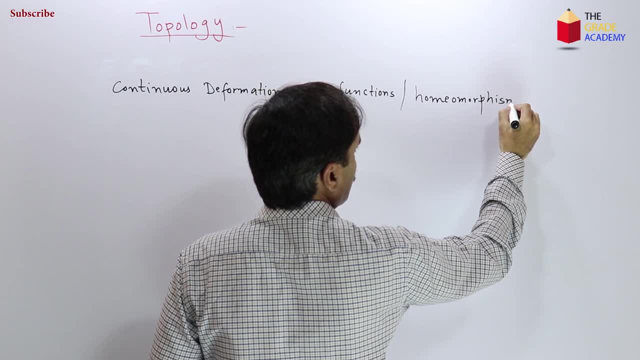 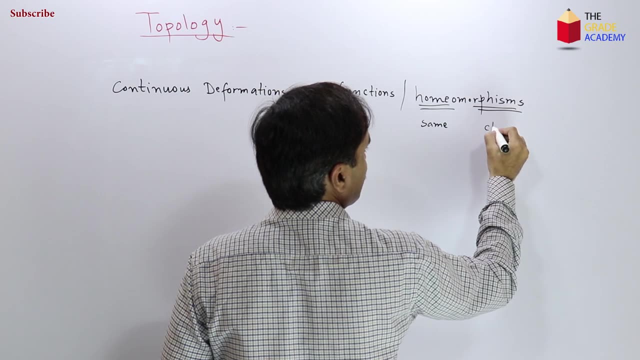 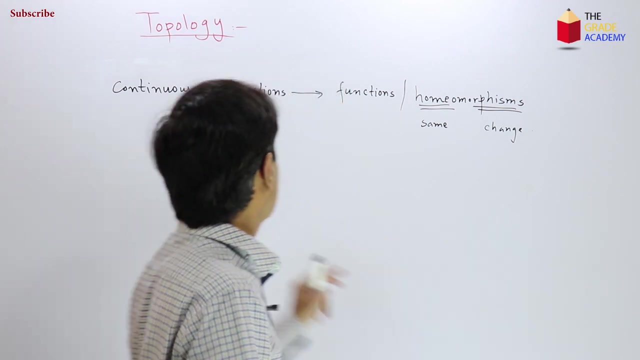 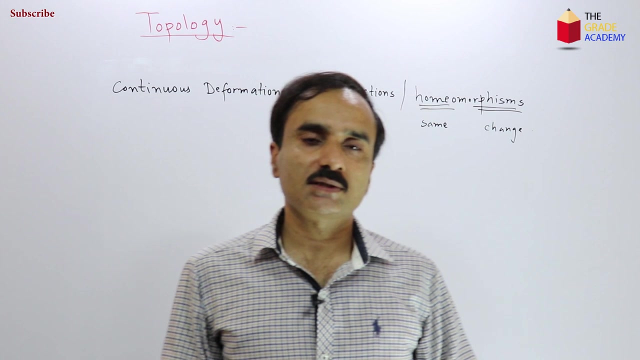 and these functions are called homeomorphisms. Homeo means same and morphism means change. deformations in topology are functions which are called homeomorphisms, and the objects which are obtained as a result of continuous deformations they are called homeomorphic. 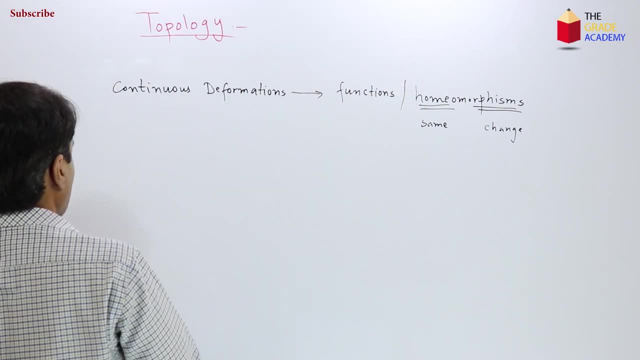 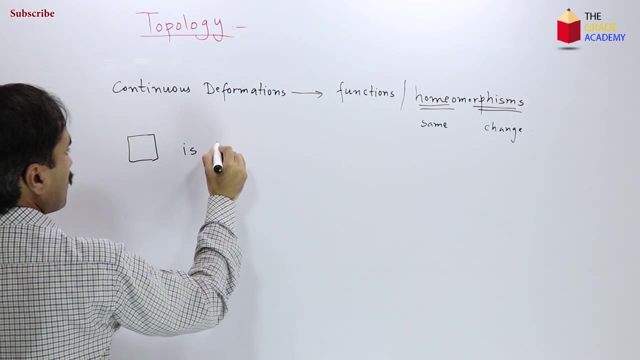 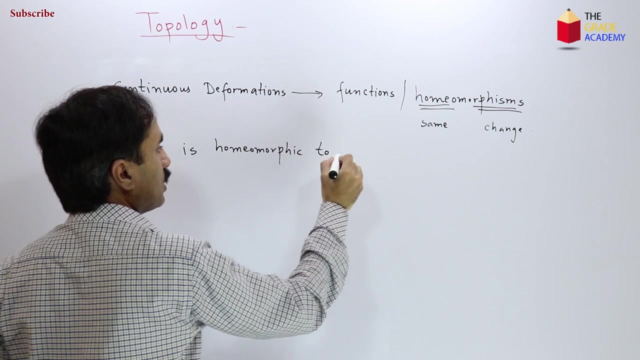 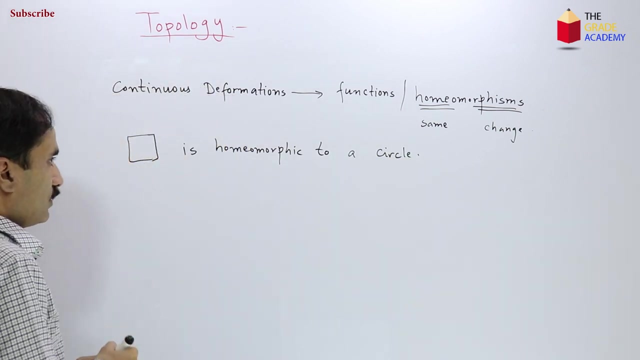 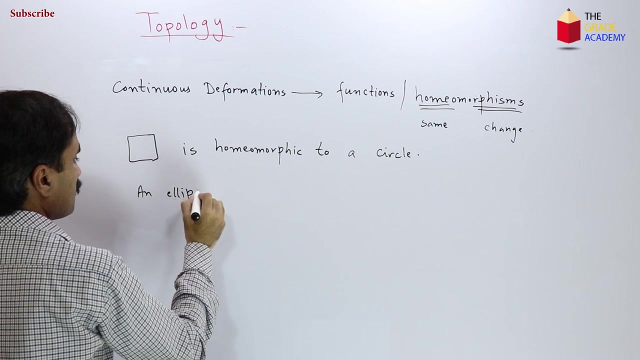 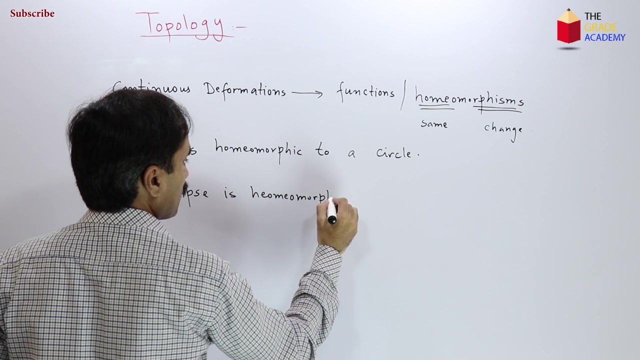 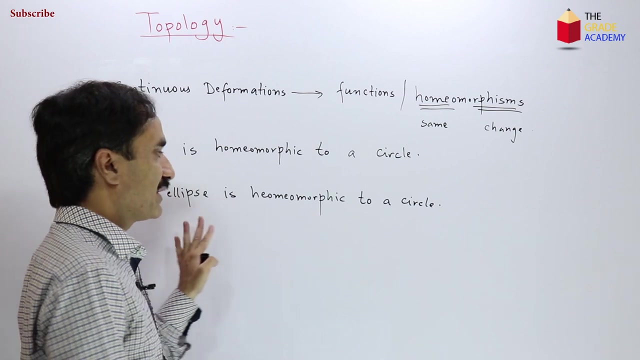 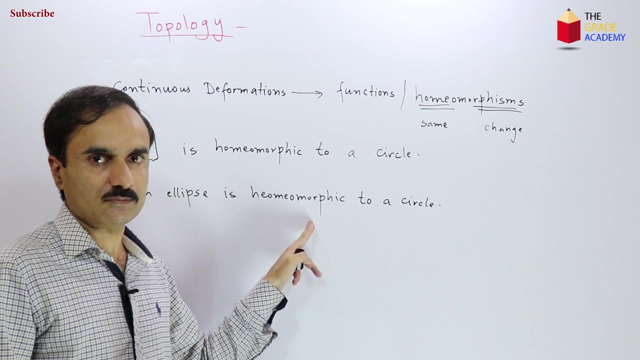 to each other. So a square is homeomorphic to a circle. similarly, an ellipse is homeomorphic to a circle, Because we can obtain an ellipse by just stretching a circle. So they are topologically the same, or they are homeomorphic because one can be obtained from another by a continuous deformation. 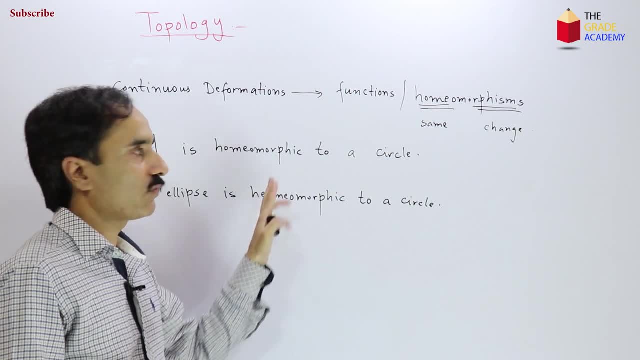 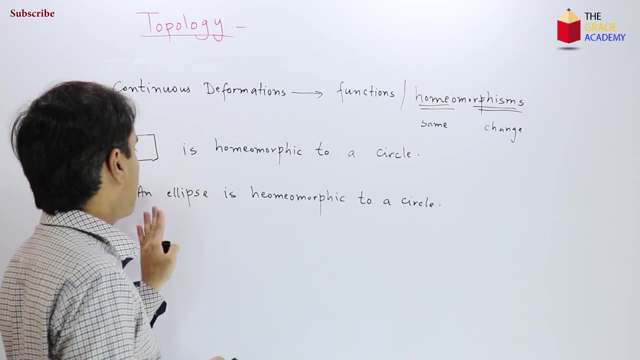 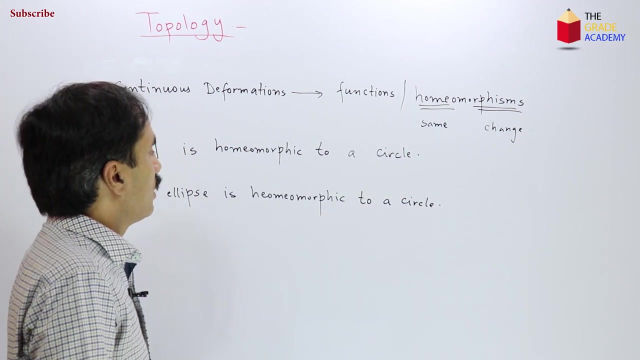 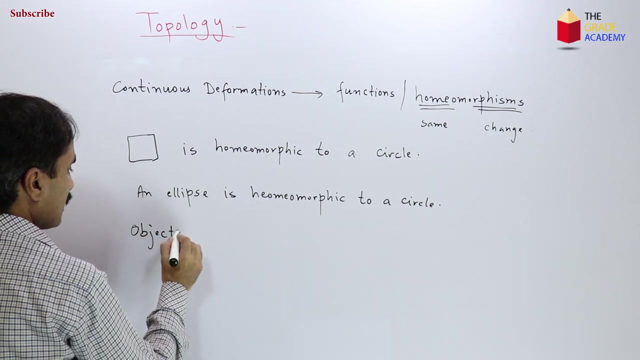 of stretching, And that continuous deformation can be obtained by a continuous deformation of stretching, and that continuous deformation is what we call homeomorphism in topology. So hence, square is homeomorphic to a circle and an ellipse is homeomorphic to a circle. And the objects and objects that we consider in topology under homeomorphism- and they are- 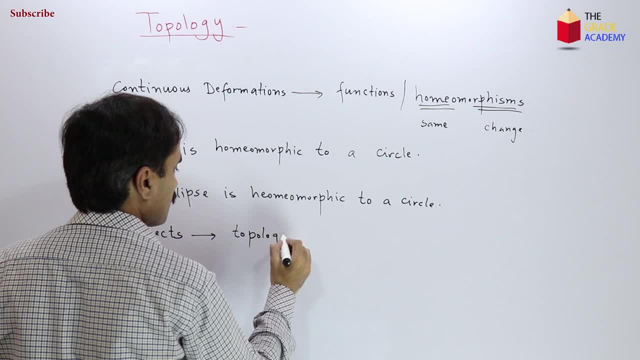 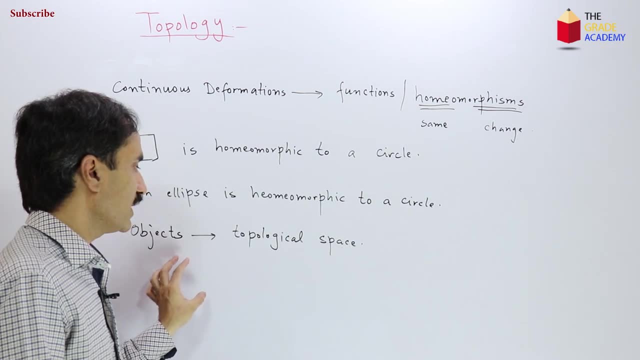 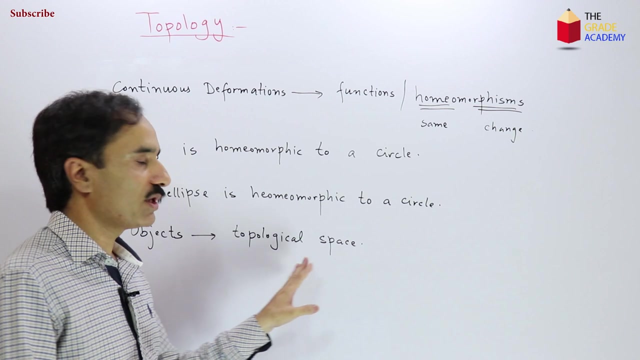 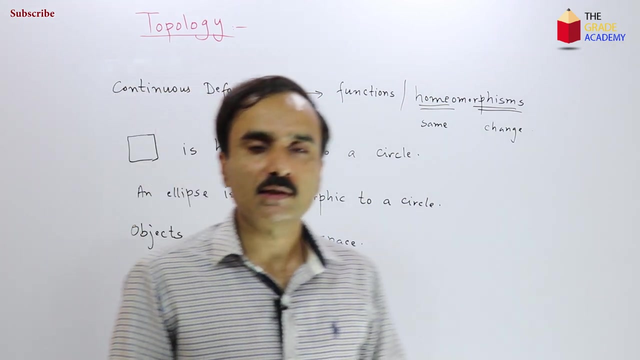 typically topological spaces, So the objects that we consider in topology. they are called topological spaces, As we will see in the upcoming lectures, that a topological space is a kind of a group or a set. So topology basically studies shapes as groups or sets, So it does not exist in 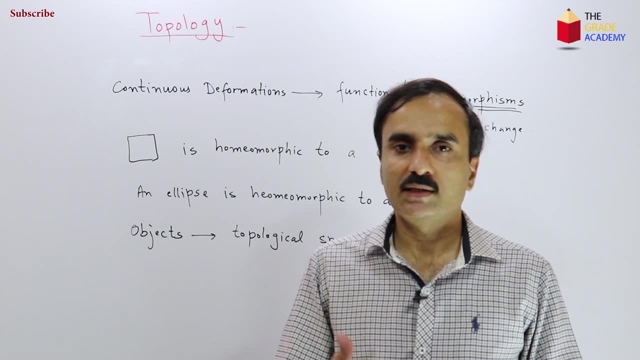 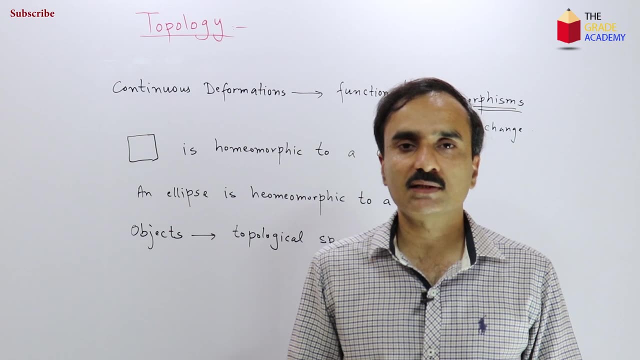 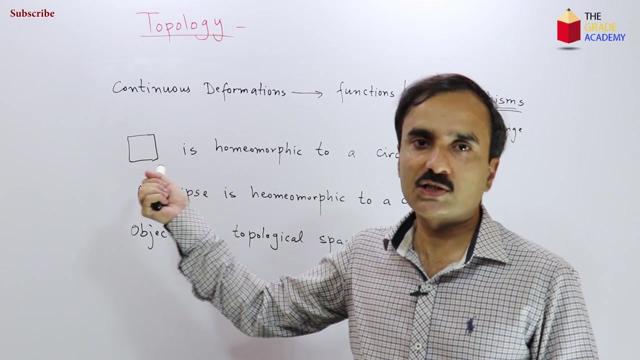 the topological space, So it does not exist in the topological space as we know that. So it does not exist in the doesn't care about the length and volume and angles. that is why in topology all the triangles are the same. similarly, as we just saw, that a square is. 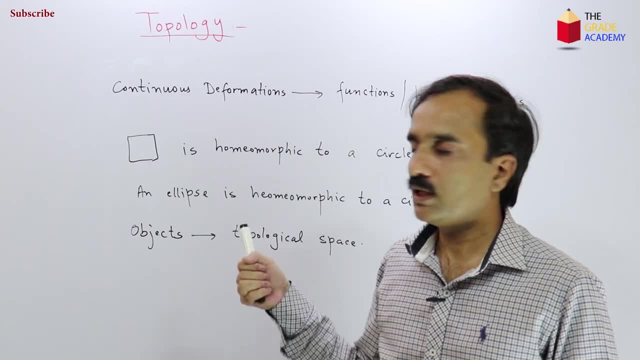 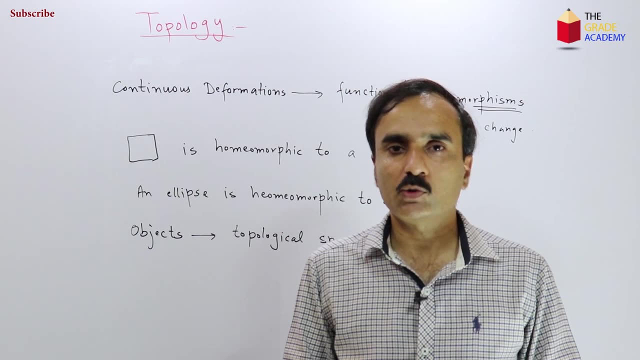 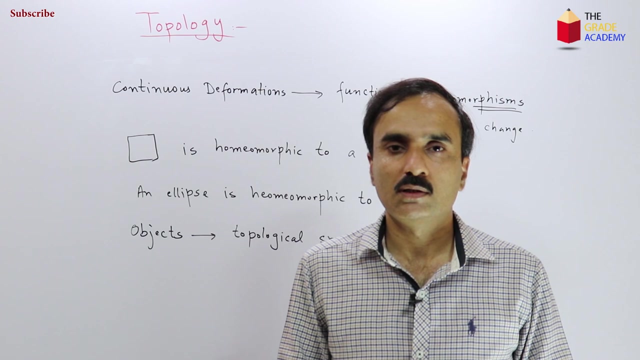 topologically the same as a circle. an ellipse is topologically the same as a circle, and there is a famous joke in mathematics that a topologist is a person who cannot differentiate between a doughnut and a coffee cup. so a doughnut and a coffee cup basically are continuous deformations of one another. 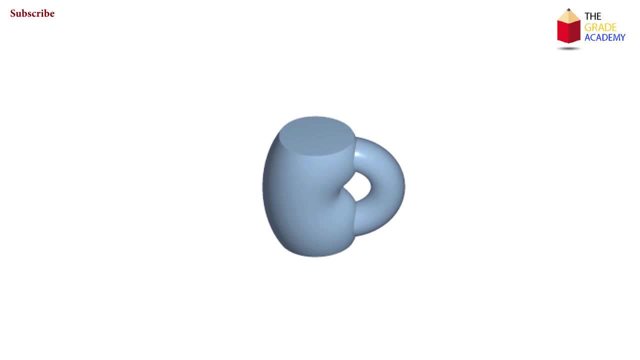 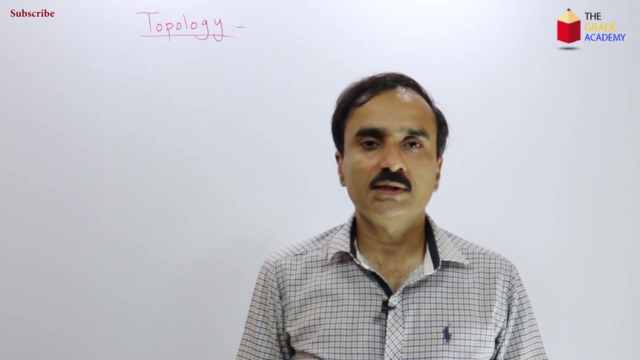 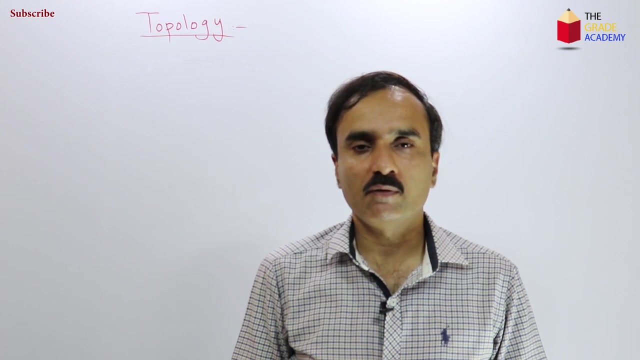 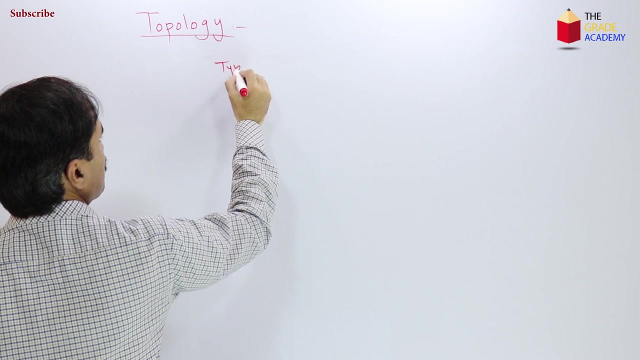 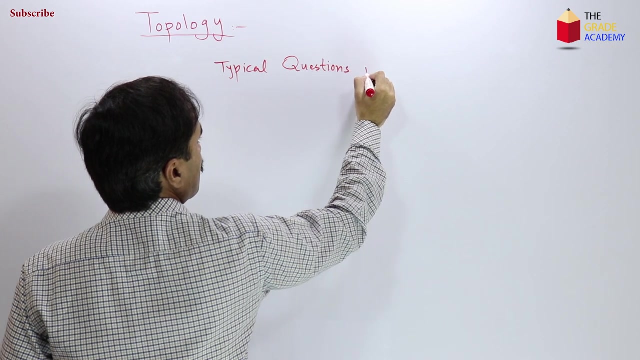 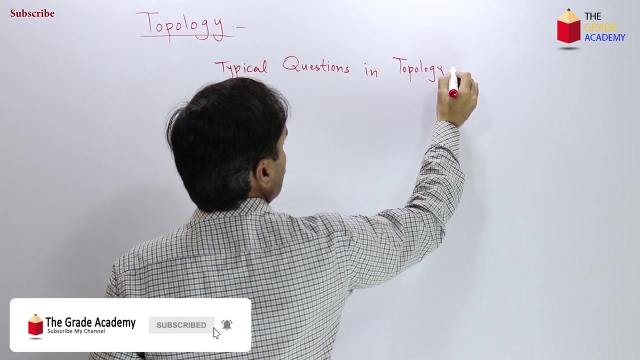 so they are topologically the same, they are topologically equivalent or they are homeomorphic to each other. now we will see some of the typical questions that we will be working around throughout this video about our study of topology, and these questions are so typical questions in topology. 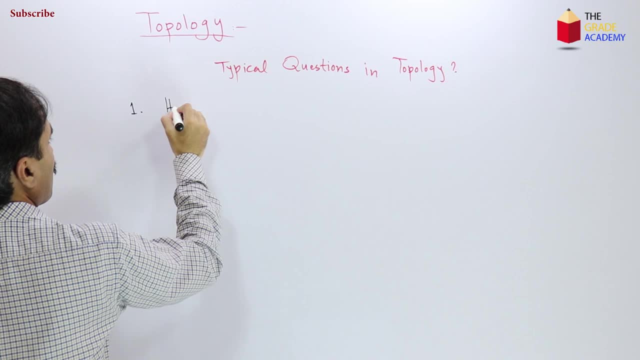 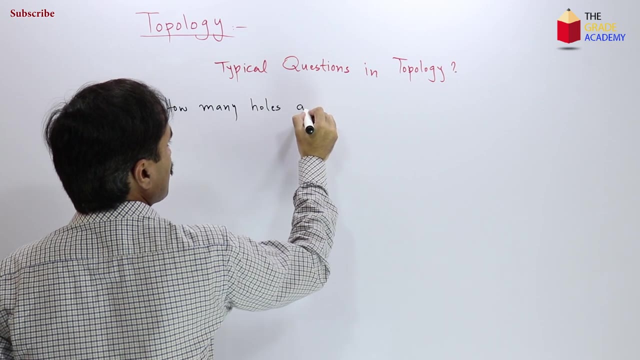 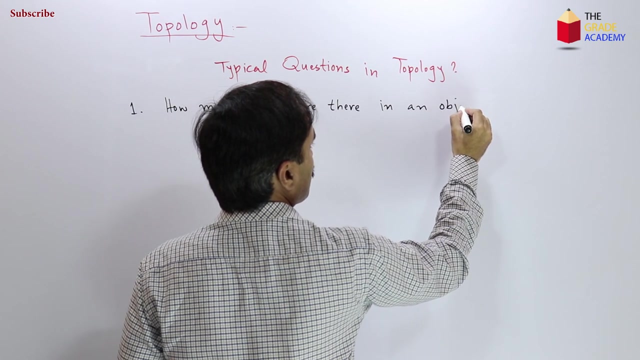 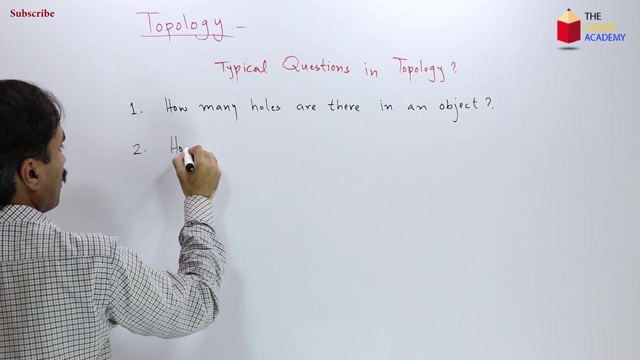 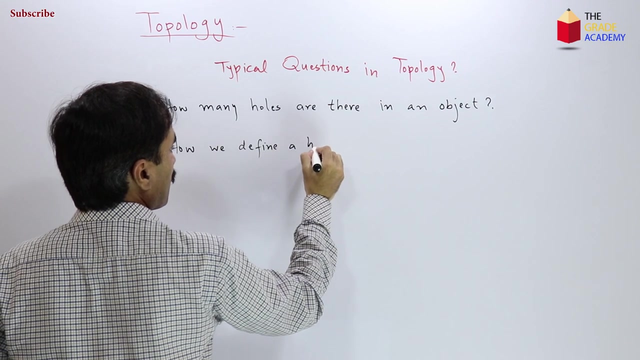 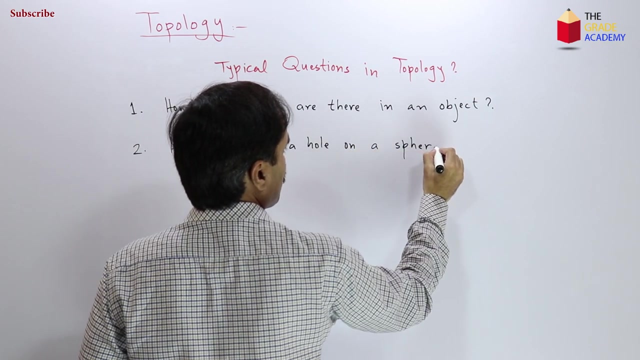 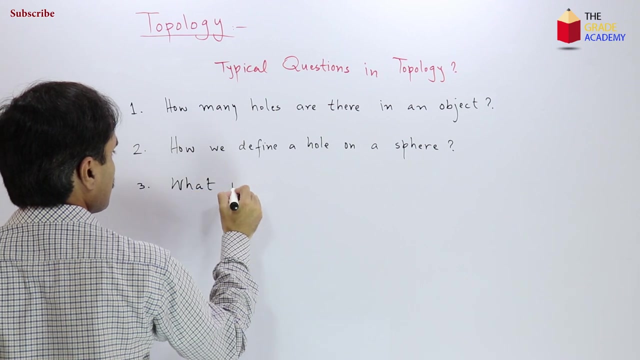 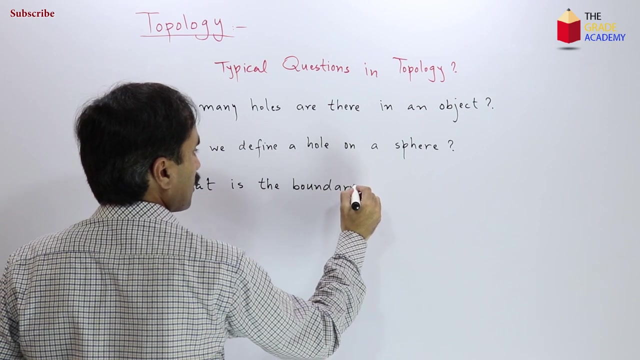 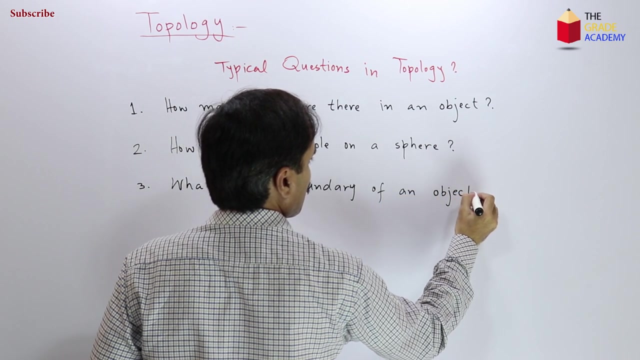 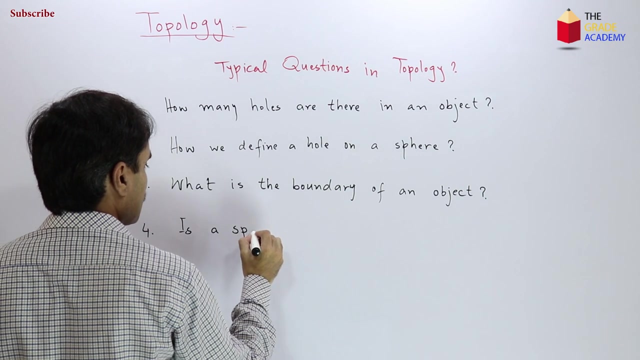 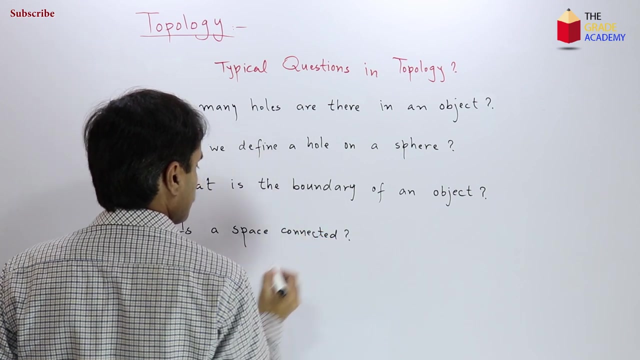 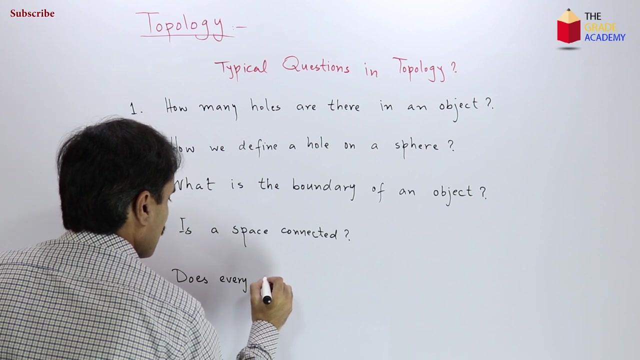 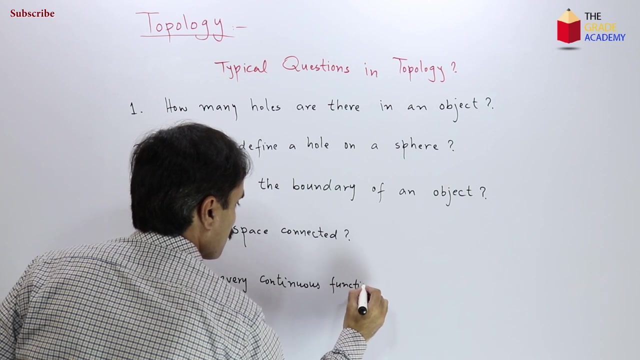 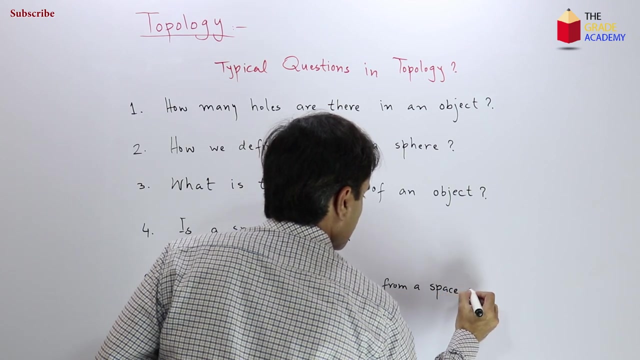 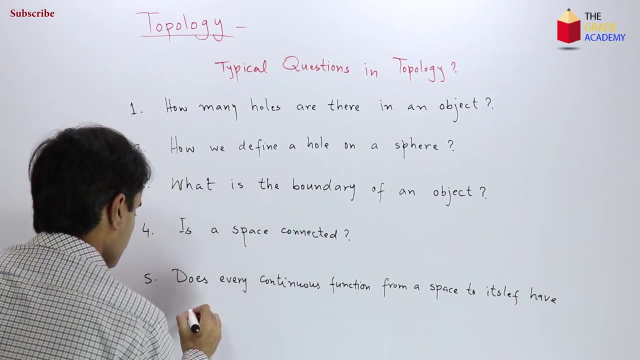 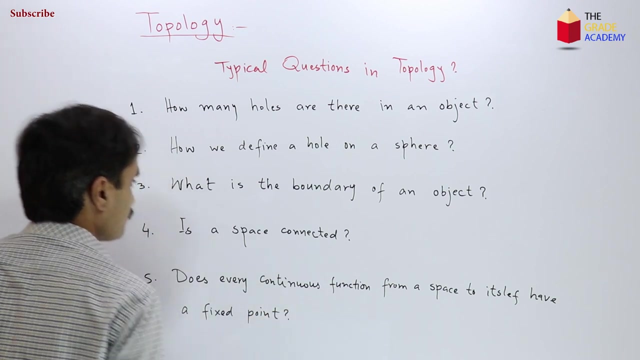 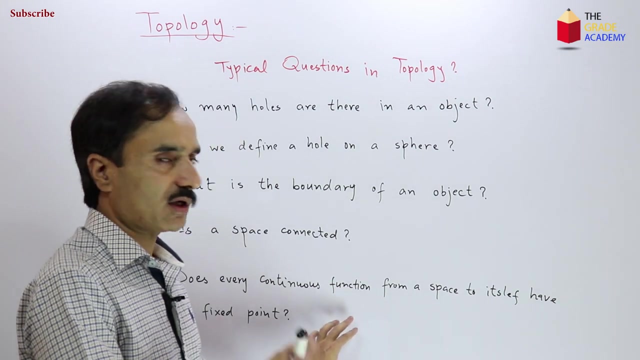 so, for example, how many holes are there in an object? and the question like how we define a hole on a sphere? what is the boundary of an object? is a space connected? so does every continuous function from a space to its cell have a fixed point? so these are some of the questions that we have to work around throughout our course.